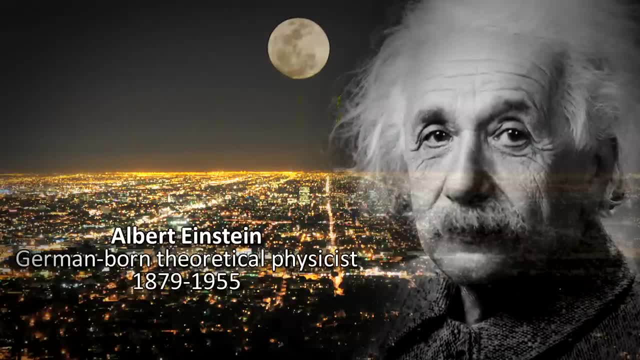 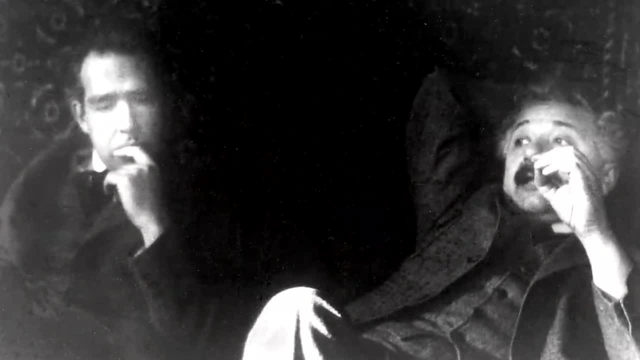 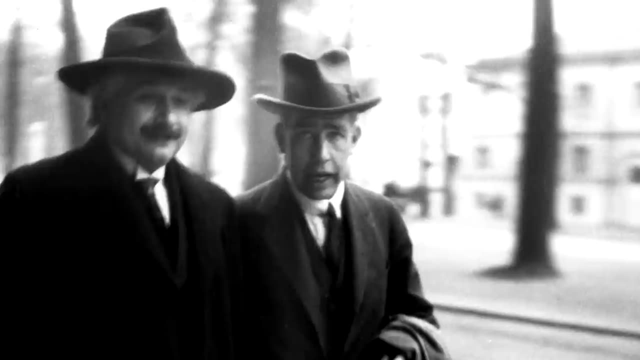 of measurement. He famously said in his dramatic statement: do you really believe the moon only exists when you look at it? Bohr and Einstein argued passionately about their views on the essence of reality and for 30 years both views were considered equally valid, and scientists 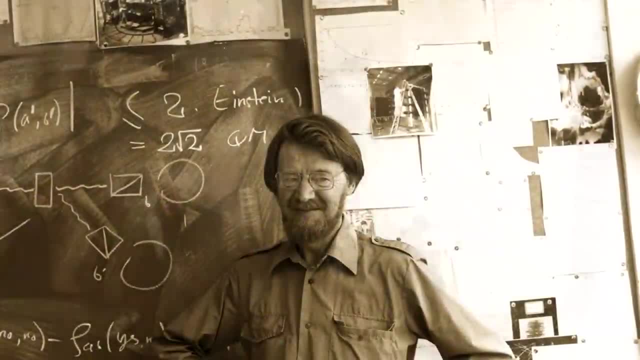 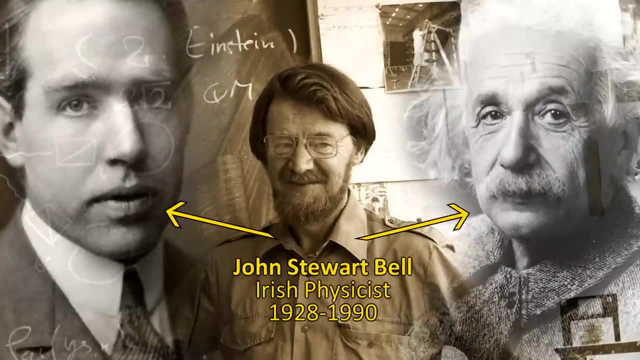 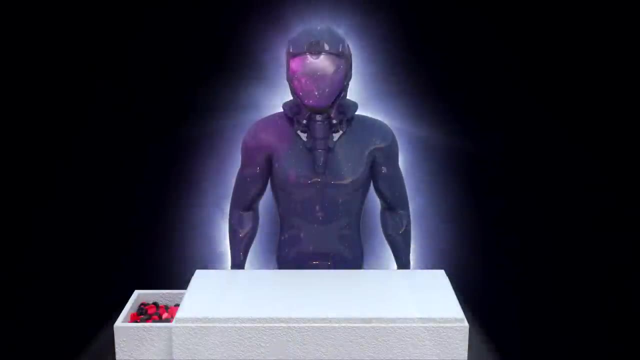 chose science. In 1964, Irish physicist John Bell devised a way to prove whether Einstein's view of a classical deterministic view of reality was correct. He put this in a simple, elegant equation called the Bell Inequality. Although the equation is simple, understanding what it means is not so easy. So how? 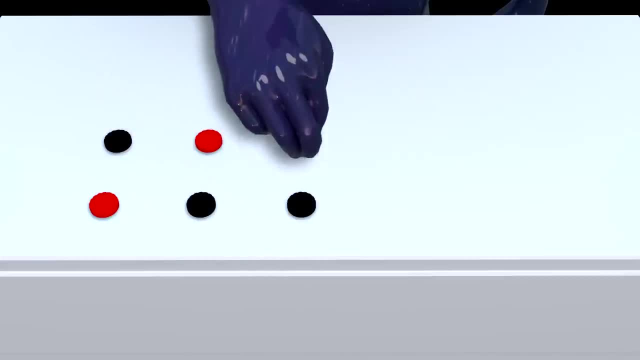 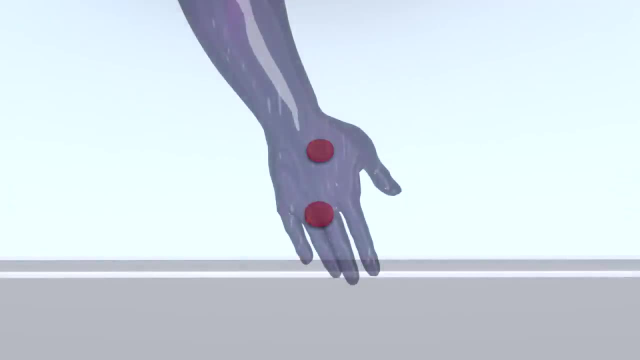 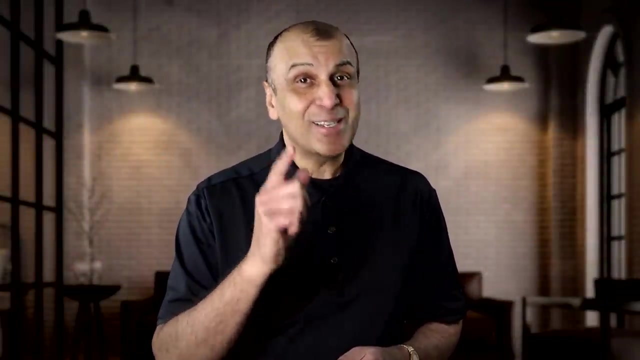 did this simple equation disprove the ideas of the most famous and powerful scientists of the 20th century and, furthermore, the most intelligent scientists of the 20th century, And forced us to confront the unsettling truth that we may live in a fundamentally non-deterministic universe? The answer is coming up right now. 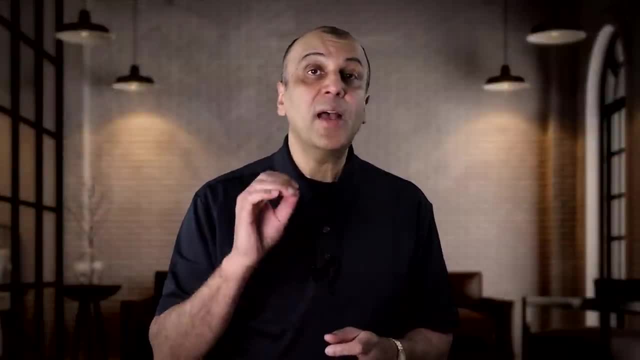 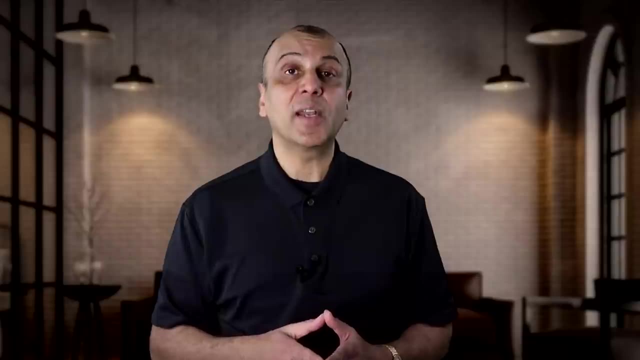 Before I talk about the EPR Paradox and Bell's Inequality, I want to point out that part of my inspiration for this video was from a documentary that I watched on Magellan TV by Jim Al-Khalili, called Einstein's Nightmare. It's a. 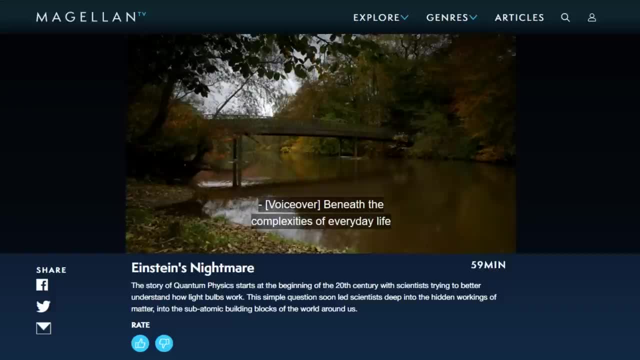 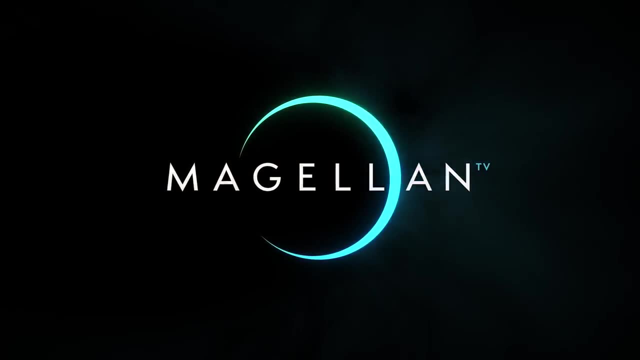 fascinating show on the full story of quantum mechanics and the thought processes that led to it becoming the defining theory of reality. This is just one of many eye-opening documentaries on Magellan TV. Magellan is a streaming documentary service that I think you're going to love. 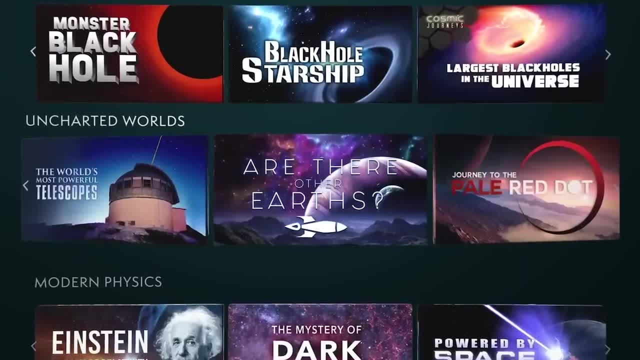 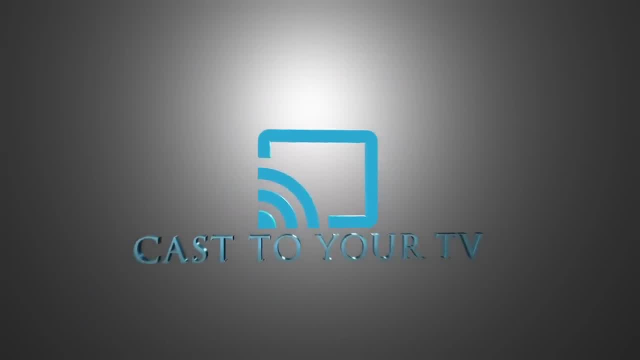 It was founded by filmmakers and producers who bring premium, in-depth documentary content. You can watch it on any of your devices as well as your TV, anytime, without any disruptions, And you can watch it in 4k. my friends, I'm dealing with the EPR Paradox and Bell's Inequality. I'm 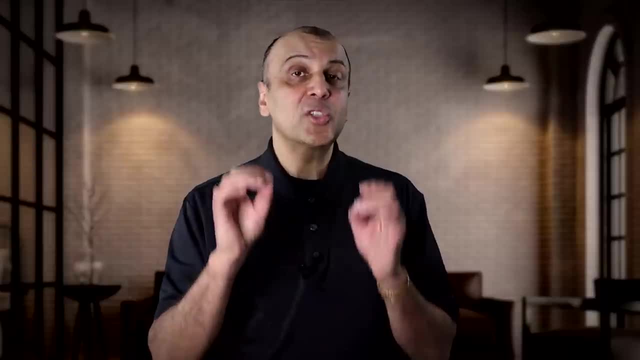 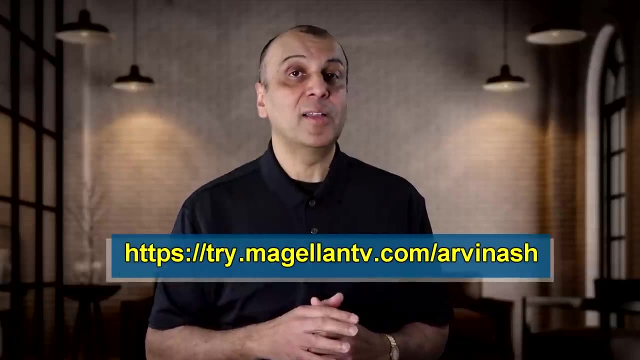 going to talk about the EPR Paradox and Bell's Inequality. I'm going to talk about Einstein's Nightmare. I'm delighted to tell you that Magellan TV has an exclusive offer right now for Arvin Ash viewers. If you use the link in the description, you'll get one free month trial. I highly recommend. 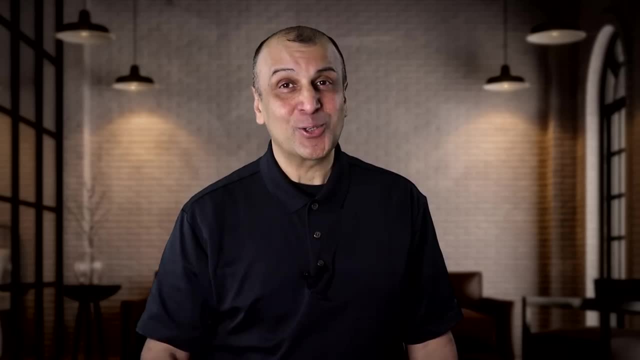 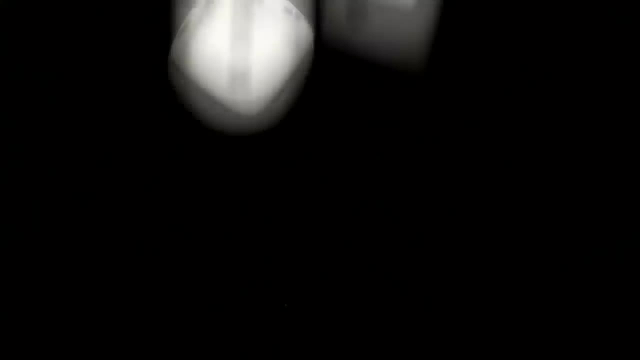 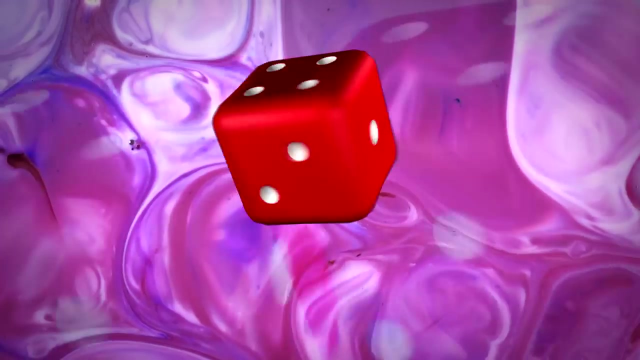 Magellan TV, but be sure to use the link in the description. The central weirdness of quantum mechanics can be demonstrated with the toss of the dice. If the dice was a quantum system like a photon, electron or atom, it would be in superposition. That is its position and other. 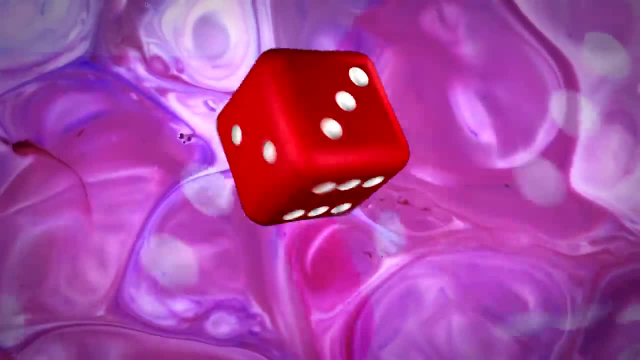 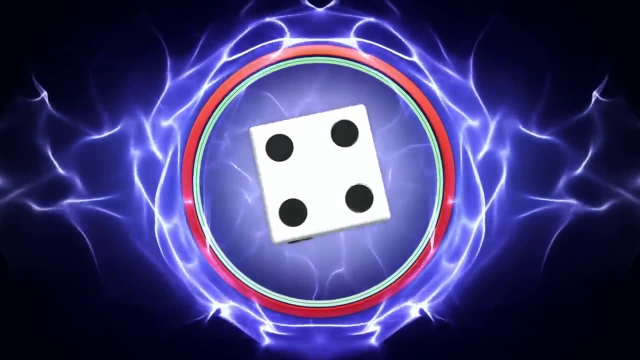 properties, in a sense, would be up in the air like a dice thrown before it hits the table. It's a 1,, 2,, 3,, 4,, 5, and 6 all at the same time, According to the most accepted interpretation of. 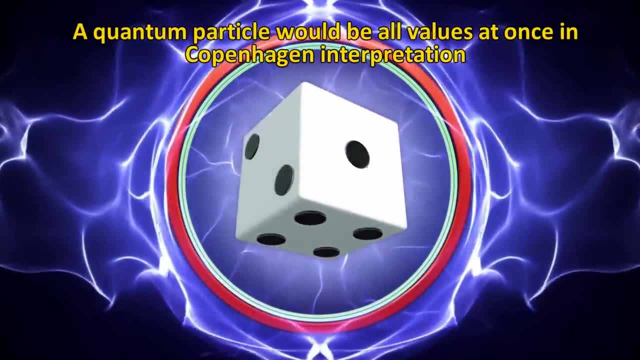 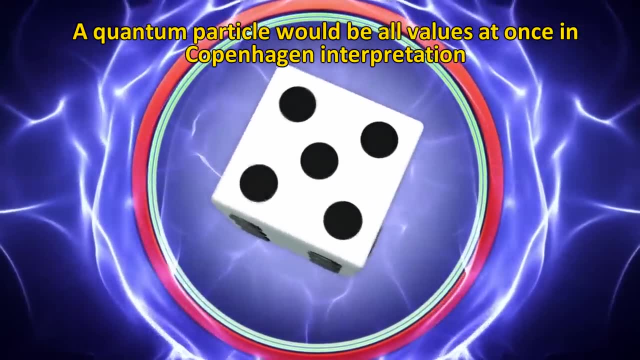 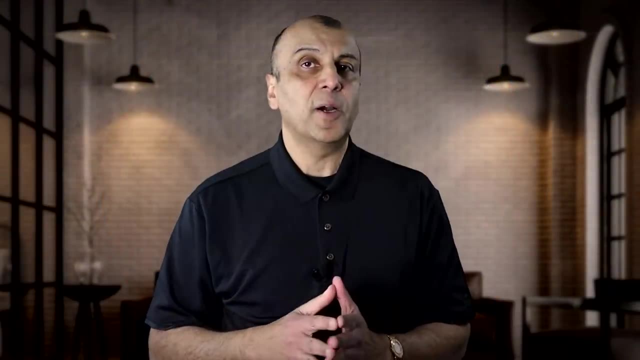 quantum mechanics. the Copenhagen Interpretation, pioneered by Niels Bohr and Werner Heisenberg. it's not only that the dice's value is not known, but that it is all values at once. Its value can only be known once it is measured. The double slit experiment. 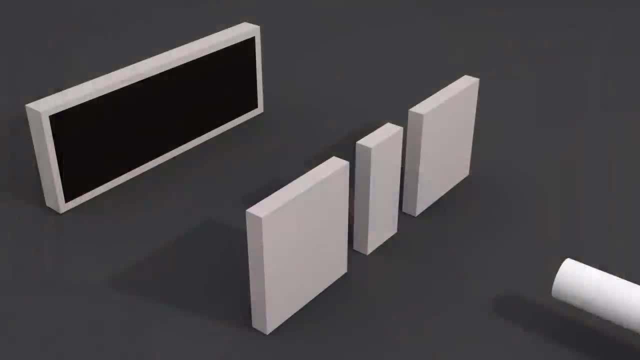 a single photon passing through the slit should not be thought of as a particle going through and interacting with itself. Rather, it's like a three-dimensional wave or cloud of probability. when it is emitted, This wave can go through both slits at once and interfere with itself. 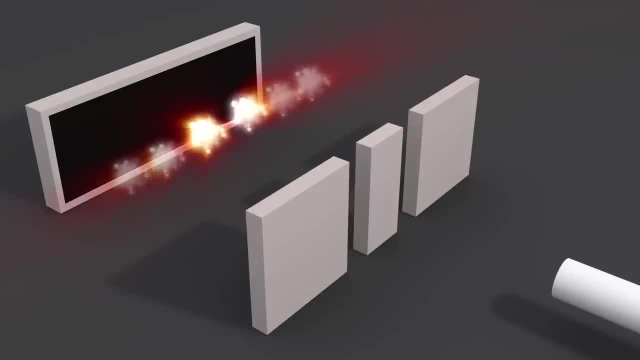 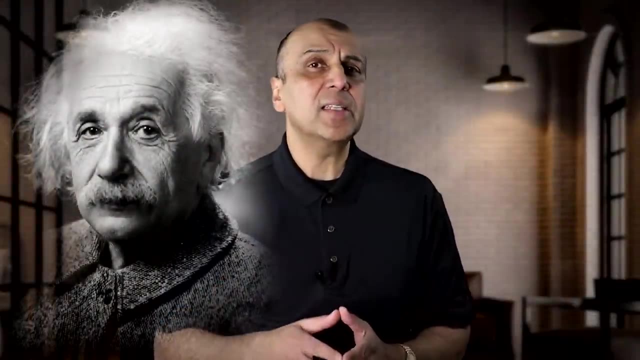 like a wave does before it is measured by the photosensitive screen in the back, when it resolves to a specific location on the screen. Einstein, who was the most famous scientist at the time, was bothered by this interpretation of quantum mechanics: The idea that part of nature 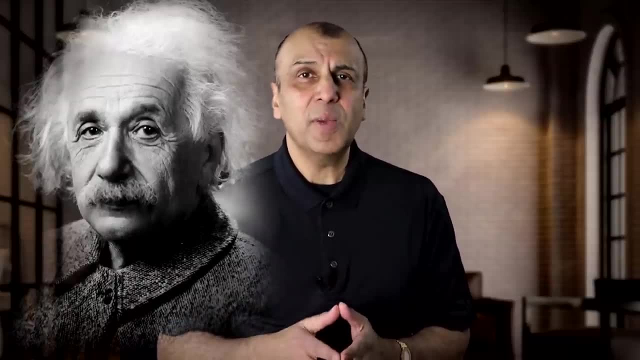 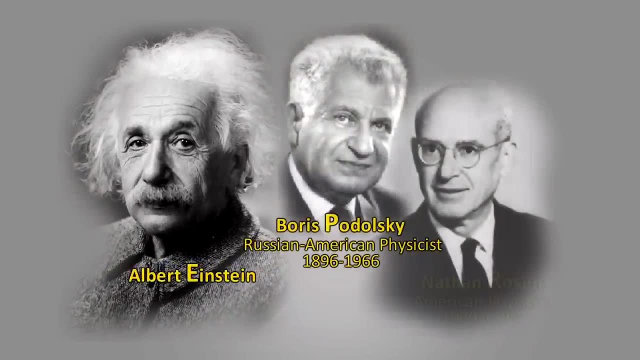 remains not only unknown, but is unknowable unless measured. That's why he famously said: God does not play dice. So Einstein, along with two other scientists, Boris Podolsky and Nathan Rosen- EPR for short- came up with what they thought disproved the Copenhagen Interpretation. 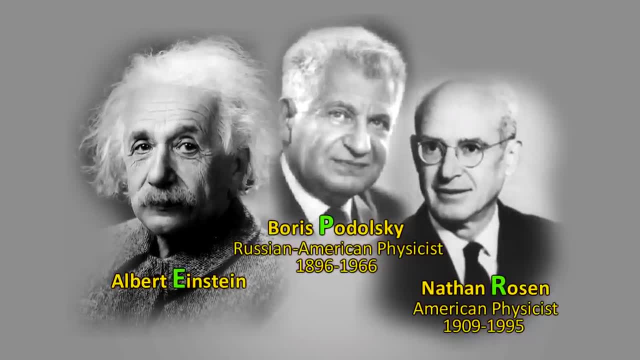 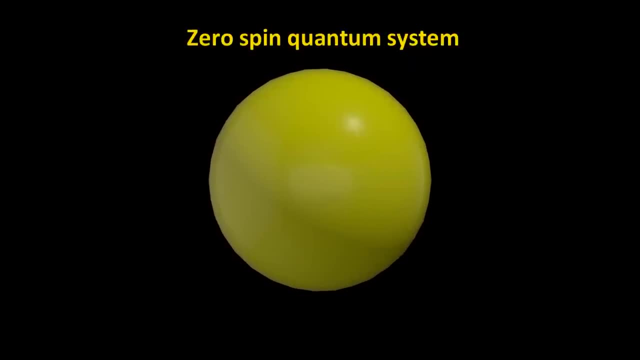 The crux of their argument rested on the idea of a phenomenon predicted in quantum mechanics called entanglement. Let's say we have a quantum system that has zero angular momentum, also known as spin zero, and it emits two photons simultaneously. Since photons have spin and since 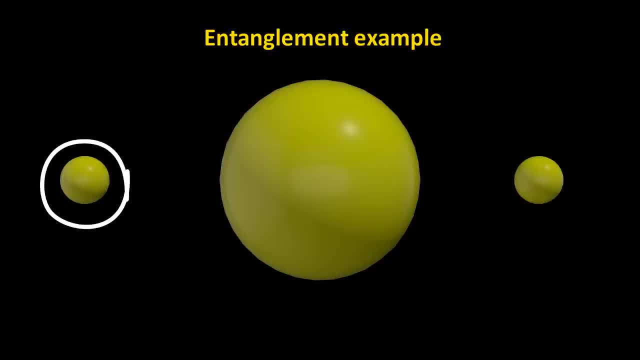 angular momentum must be conserved. if one photon has a spin up, the other photon must have a spin down. So the spin up and down cancel each other out. This is entanglement. The two photons are not independent If the spin of one of them is known. 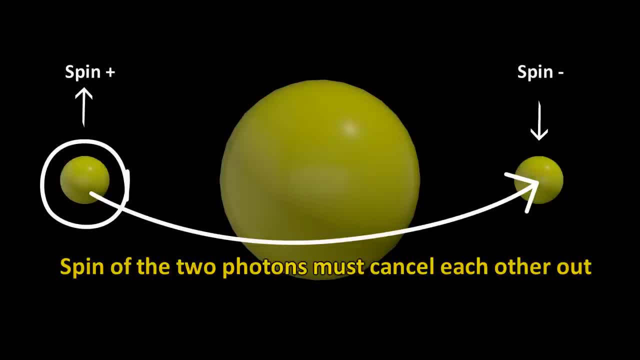 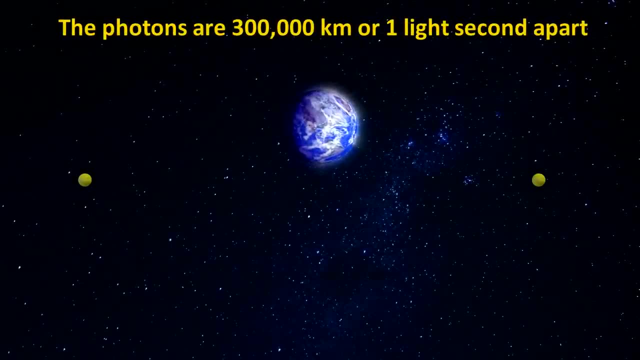 the spin of the other becomes known instantaneously. Now let's separate these photons far apart, let's say 300,000 kilometers, which is about one light second away. Now, according to quantum mechanics, each of these photons is governed by a wave function. 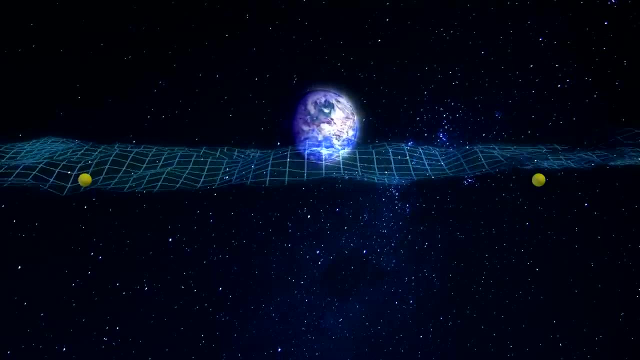 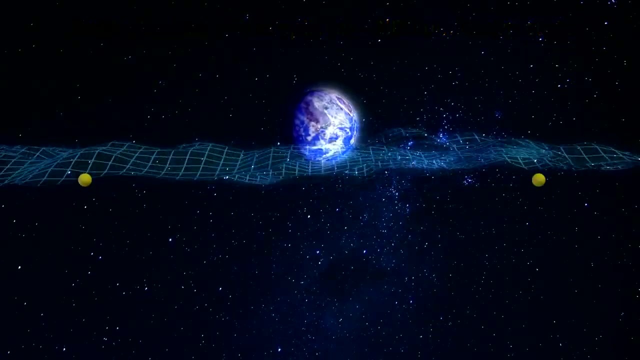 And each photon is in a state of both spin up and down at the same time. It is not up or down, it is both up and down. However, the wave function of these photons is not independent. They are really the same wave function. 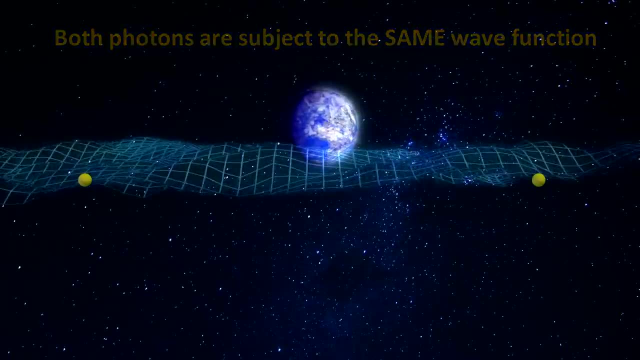 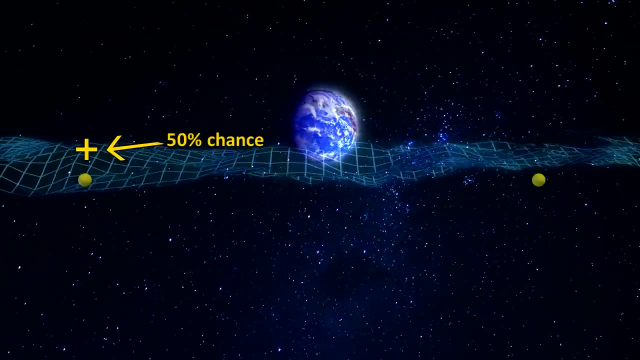 governing both photons. Now if we measure the spin of one of them, we have a 50% chance of detecting a spin up. Let's say we do detect spin up. Now let's measure the spin of the other photon in less than one second. It should also have a 50% chance of having spin up or spin down. 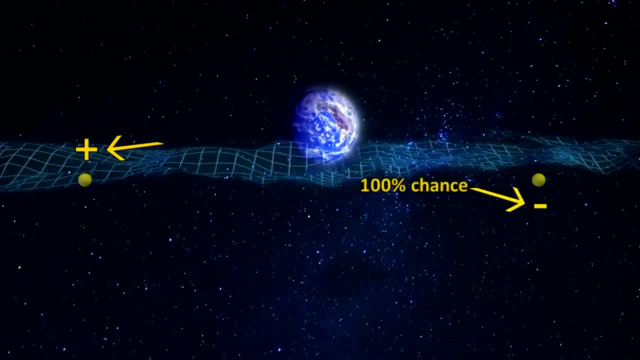 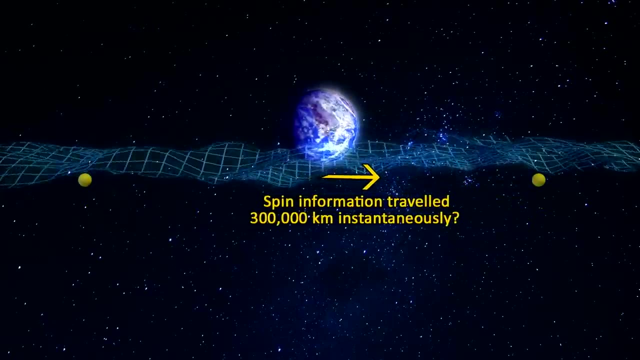 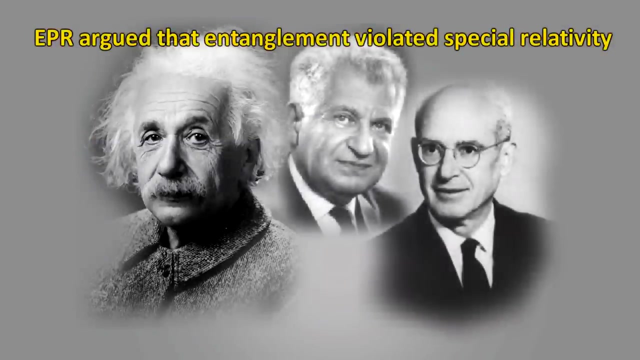 but it doesn't. It has a 100% chance of having a spin down. This means that the information of the collapse of the wave function of one of the photons had to travel faster than light to affect the other photon. EPR argued that since nothing can travel faster than light, according to the rules, 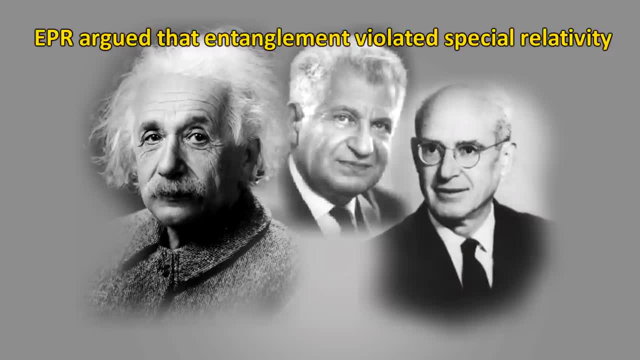 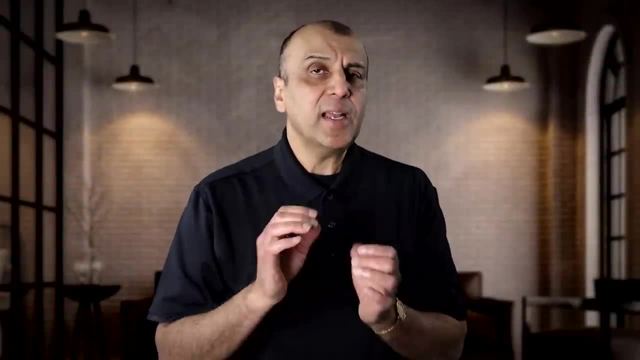 of special relativity. this should invalidate the Copenhagen interpretation. This theorized violation is the EPR paradox. EPR proposed instead that there is likely another theory which would show that the two entangled photons were in cahoots from the very beginning, that their states were. 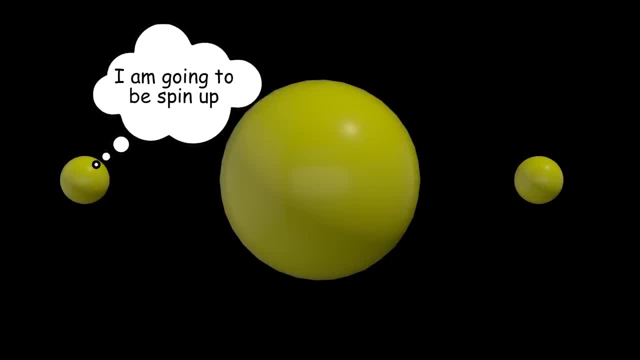 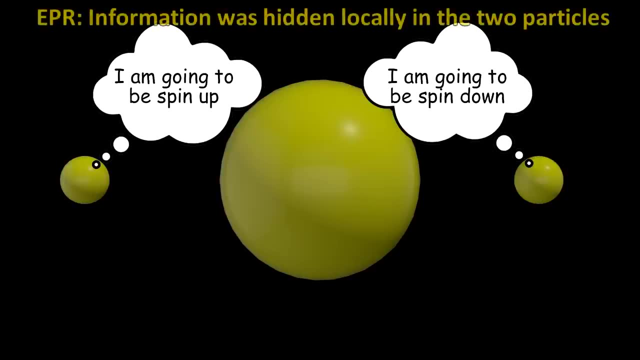 predetermined from their creation. In other words, their states contained the information locally, but when they were moved apart, no communication had to take place. The information that we were measuring was hidden inside the two particles. This is called local hidden variables. So for 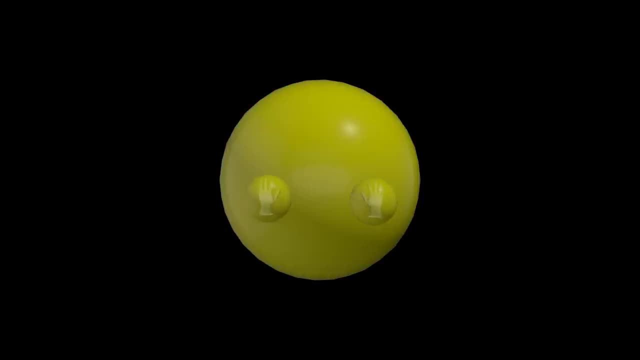 example, it's as if the two particles were a pair of gloves: One was a left-handed pair and the other was a right-handed pair. Once we found the left-handed pair, we knew immediately that the other pair, no matter where it was in the universe, must be a right-handed pair. This was a valid. 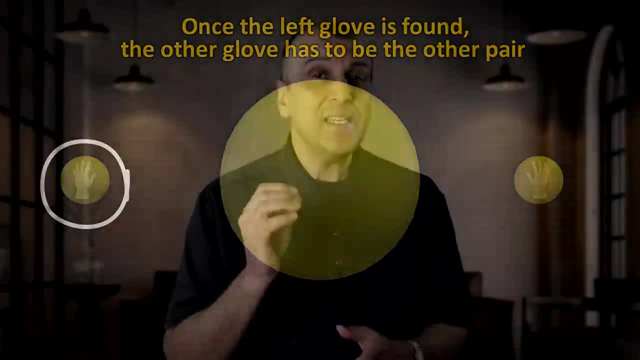 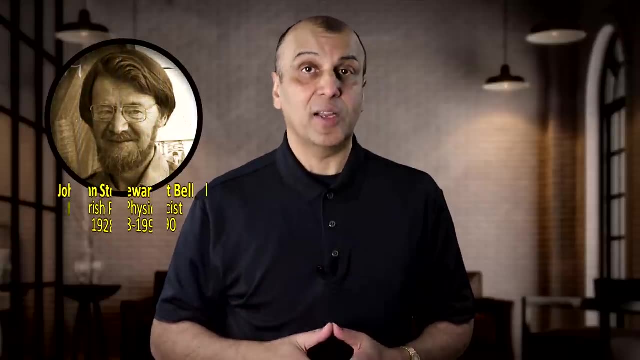 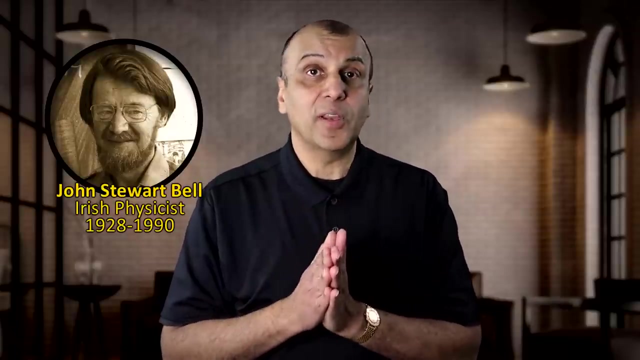 interpretation of quantum mechanics From 1935 to 1964, this could not be disproven. This is where Irish physicist John Bell comes in, And in 1964, he proposed an experiment that could show whether the local hidden variable theory was correct or incorrect. Now Bell's equation is remarkably simple, but it's one of the most 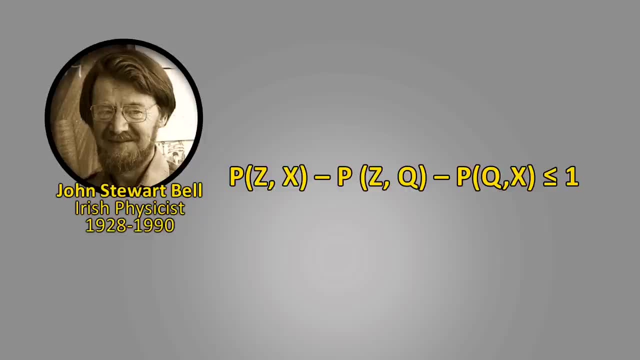 difficult to understand and simplify. So I'll present a highly simplified idea of how it works, then also show you how it works. I'll show you the simplified version of the mathematical underpinnings later in this video. Now we're going to play a game and our opponent is going to be the universe. 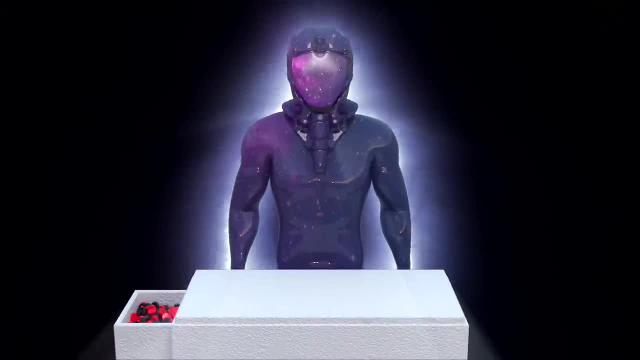 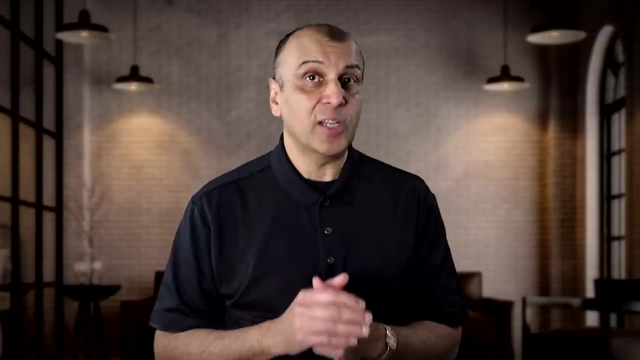 And the game is: guess the color of the checkers pieces. Now I want to give a big shout out to Jim Al-Khalili, who shows a similar simplified illustration in a documentary available on Magellan TV. I encourage you to check it out because it's fascinating If I guess the color. 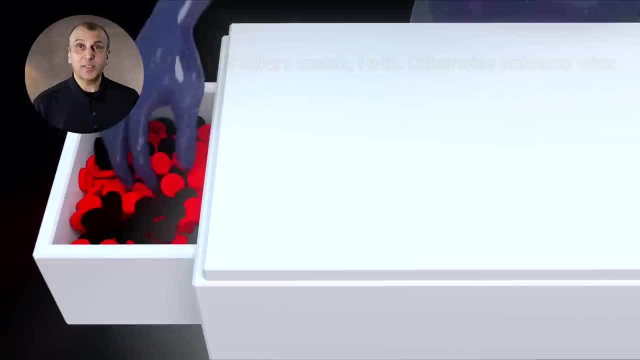 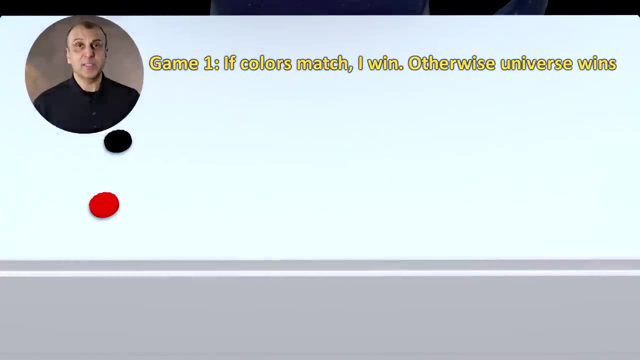 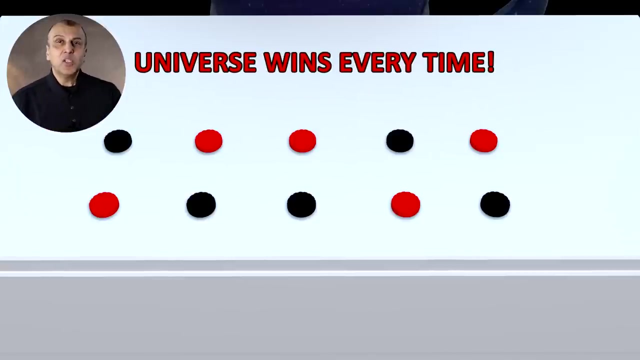 correctly, I win. If I'm incorrect, the universe wins. In the first game, I declare that if the colors match, I win. The universe picks the pieces. Now, in play after play, I find that I lose every time. So in the next round I change the rules. This time I declare that if the colors are 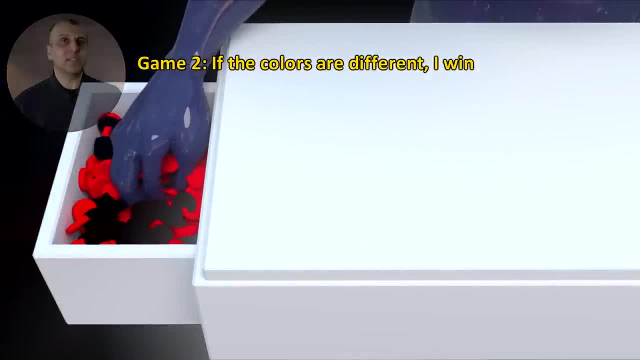 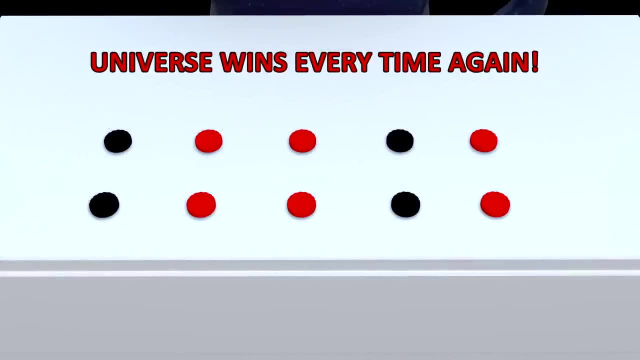 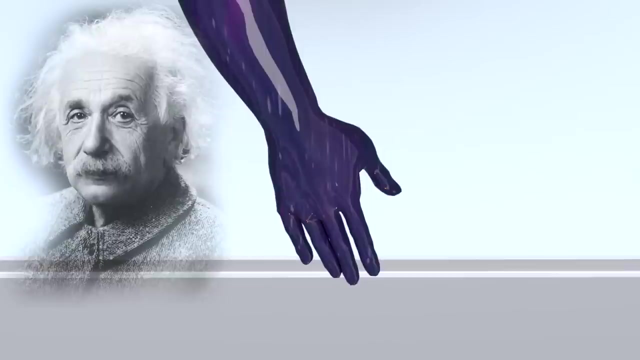 different. I win. The universe picks the pieces. In play after play I find that I lose every time again. So I conclude that perhaps the universe has rigged the game against me. Now, if I guess the color of the checkers pieces, this is some additional information that. 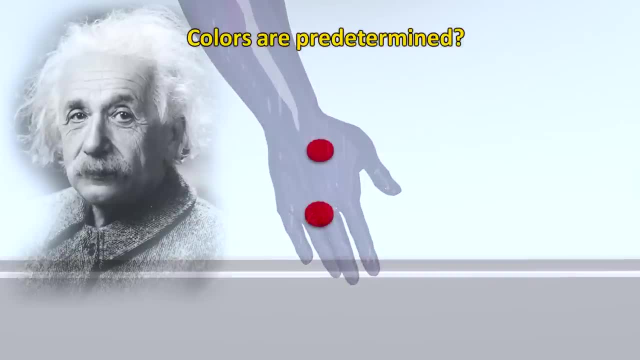 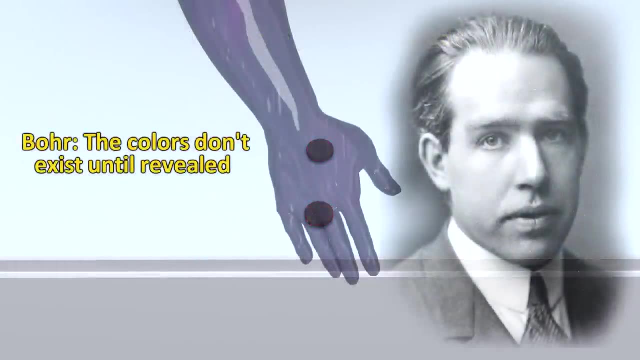 Neil Stein suspected was happening, That the checkers pieces were rigged. He believed that the colors of the pieces were predetermined and that this information had been known from the very beginning, when the two pieces were together. Neil Bohr's idea, on the other hand, was that the 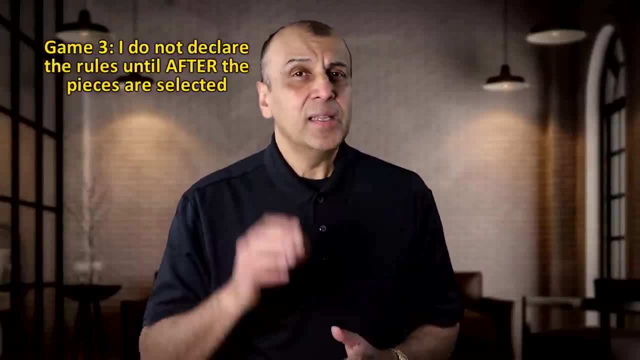 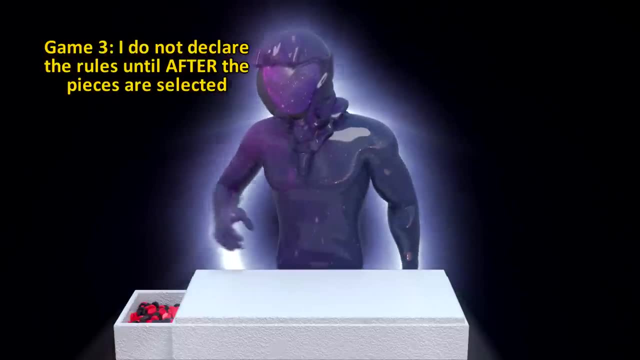 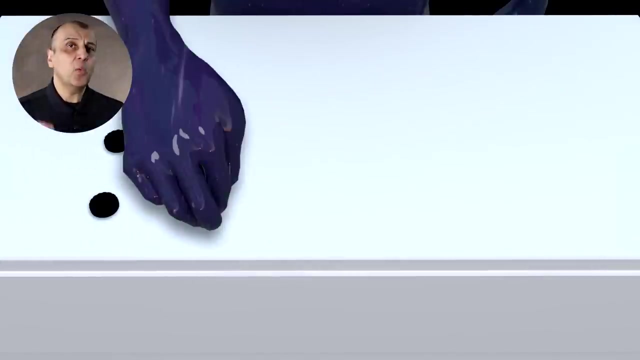 red and black don't even exist until the piece is turned over. So I changed the rules of the game again. This time I do not tell the universe whether matching colors or different colors will win the already picked, the checkered pieces. If, after revealing the checkered pieces, I find that 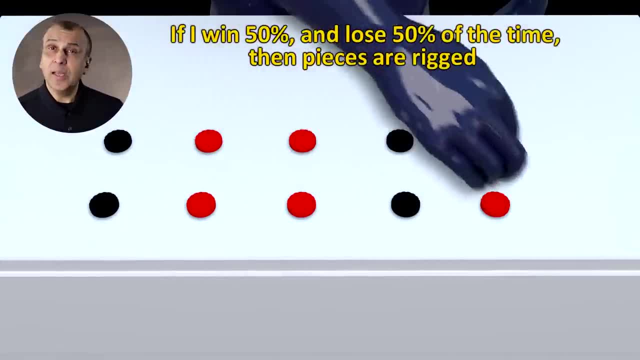 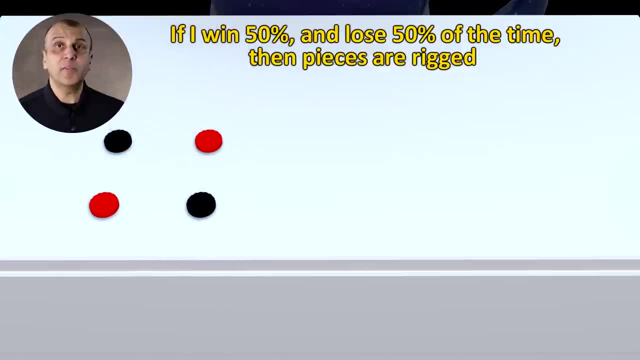 I win 50% of the time and lose 50% of the time, then my conclusion is that, indeed, the checkered pieces were rigged from the very beginning, because my chances of winning would be 50% if the red and black pieces were already picked by the universe. But if I continue, 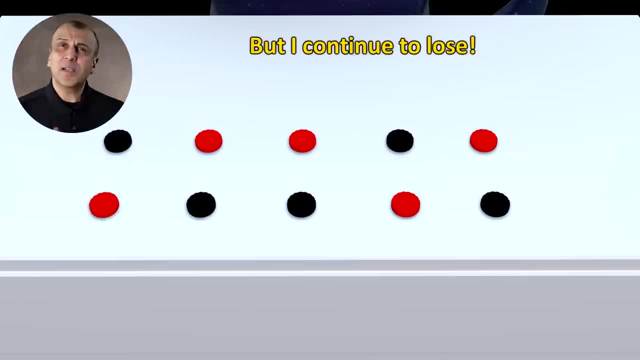 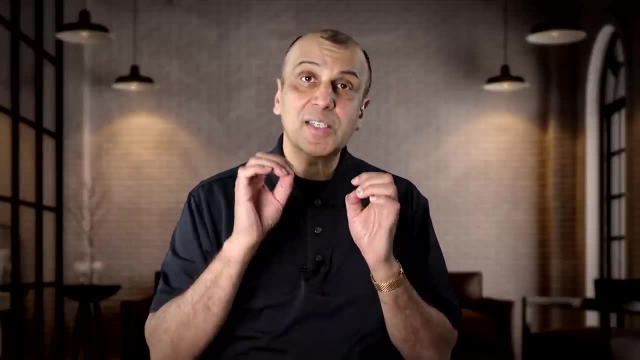 to lose, then I have to conclude that somehow the colors of the checkered pieces were not chosen ahead of time. Let's look at how Bell's Elegant Equation proves my conclusion. To do this, let's look at a universe where local hidden variables are correct. In other words, 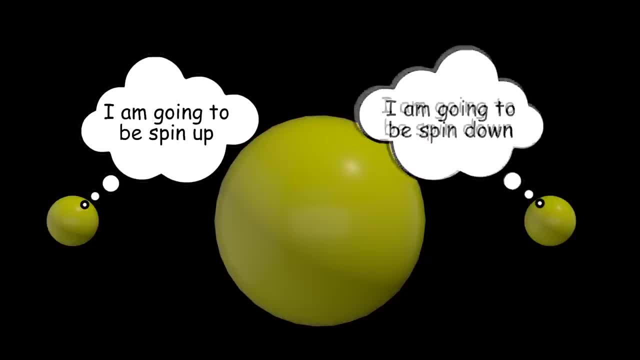 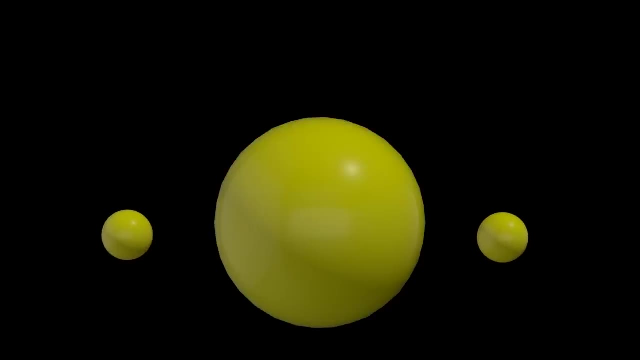 entangled particles have predetermined properties which are complementary to each other at the moment of their creation. Note that this is not an interpretation of quantum mechanics. It's an alternative to quantum mechanics. So in this system, when two entangled particles are produced from a process that conserves linear and angular momentum, we will get a. 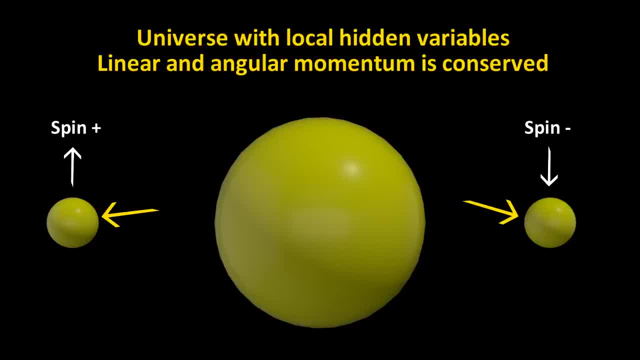 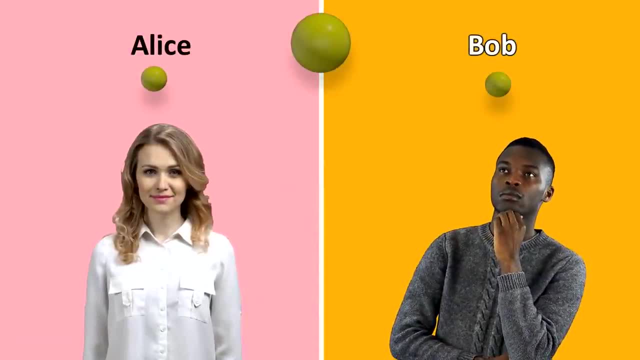 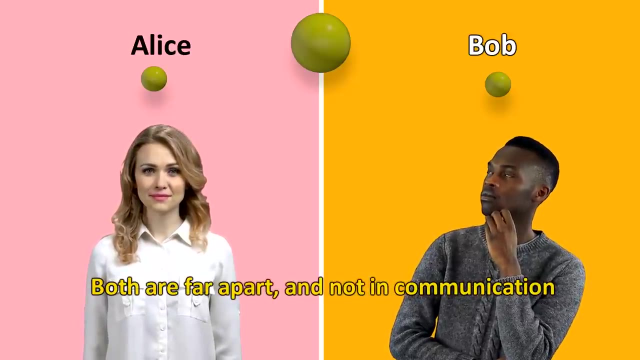 two-particles that go off in opposite directions as well as opposite spins, and they will be two opposite directions too. Let's say Alice makes the measuring on Particle 1 in her laboratory and Bob makes the measurement on Particle 2 in his laboratory, And let's say the two labs are far apart and are not. 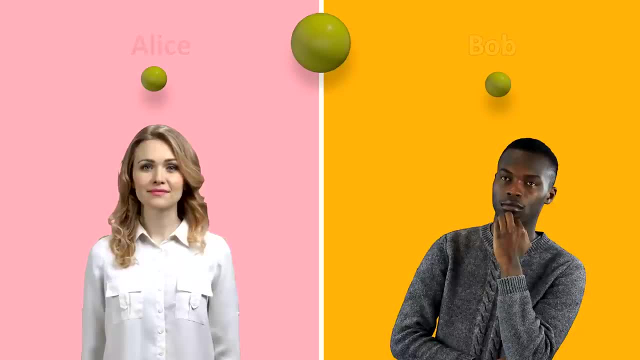 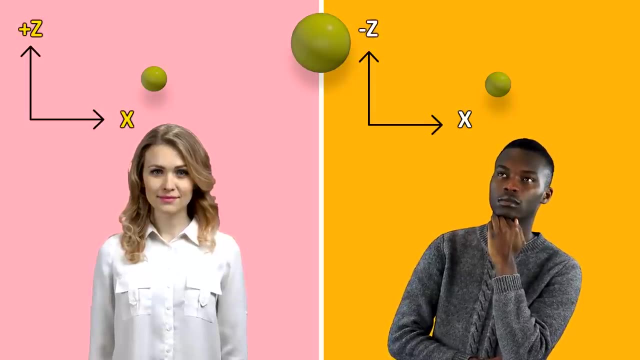 in communication with each other. If Alice measures the particle spin in the z-direction as positive or positive in particle 1, Bob will measure the particle spin as negative in the z-direction direction. If they measure the spin in the x direction, which is orthogonal to the z, 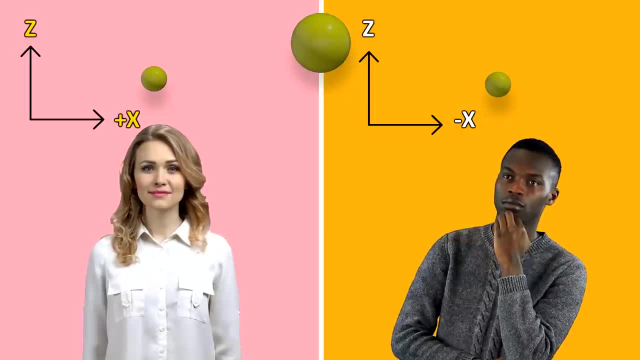 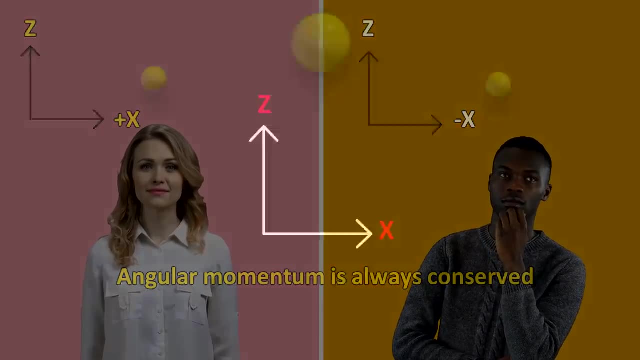 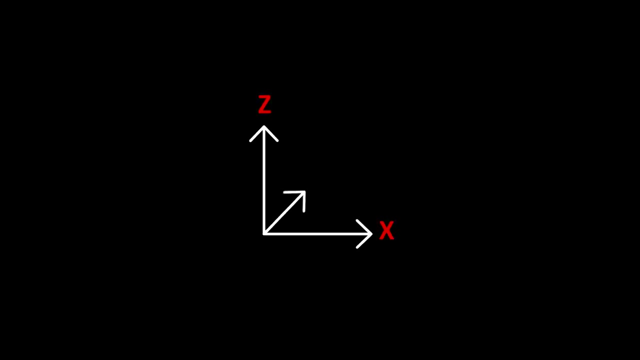 direction or 90 degrees apart, the same type of complementary opposite spins will be measured Because, as I said earlier, angular momentum is always conserved. What Bell's inequality does is it says: now let's make a third measurement. that is somewhere in between the z and x axes. In our example, if we use 45 degree angles to the z and x, 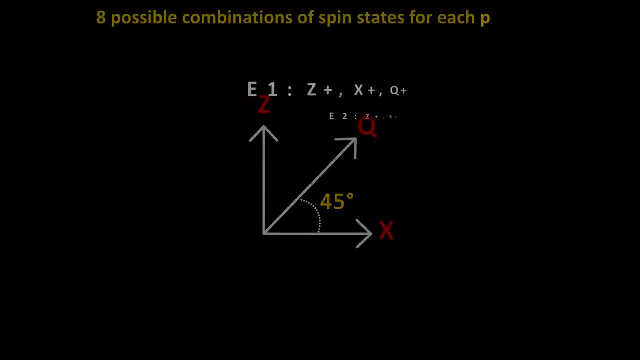 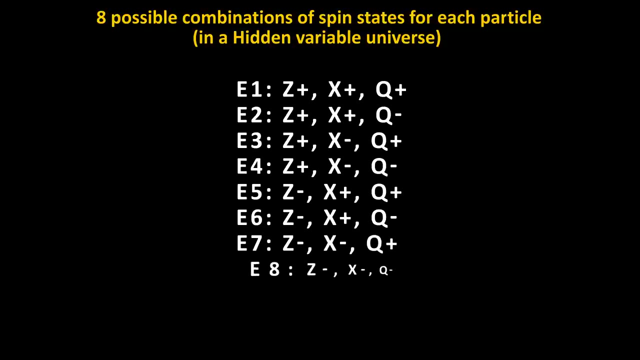 direction. we'll call this the q direction. So in a universe where local, hidden variables are true, when the two particles are emitted, they know what their state is going to be in all three directions- z, x and q- from birth, And there are only eight combinations. 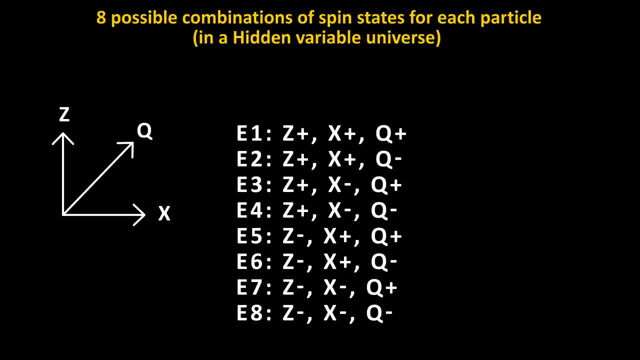 or possibilities of spins that each particle could have. So for Alice and Bob, these eight combinations will be the following: The event 1 could be where the spin in the z direction is positive, the spin in the x direction is positive and the spin in the q direction is positive. E2 is when z is positive, x is positive, 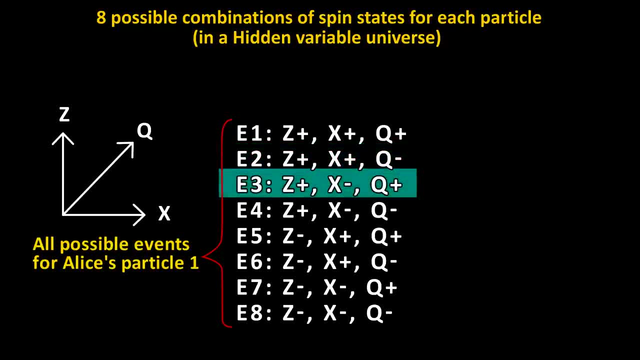 and q is negative. E3 is when z is positive, x is negative and q is positive. E4 is when z is positive, x is negative and q is negative. E5 is when z is negative, x is positive and. 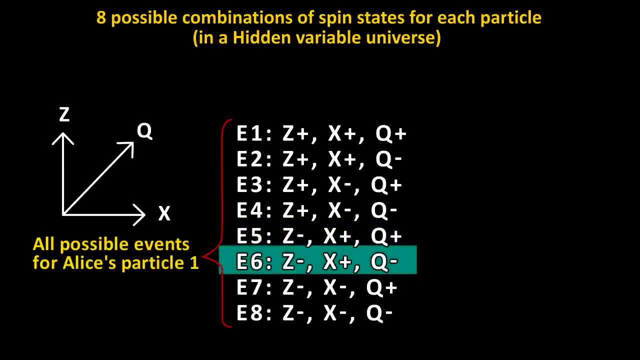 q is positive, E6, z is negative, x is positive, q is negative, E7, z is negative, x is negative and q is positive. Now let's ask the question: what is the probability that Alice measures in the z direction gets? 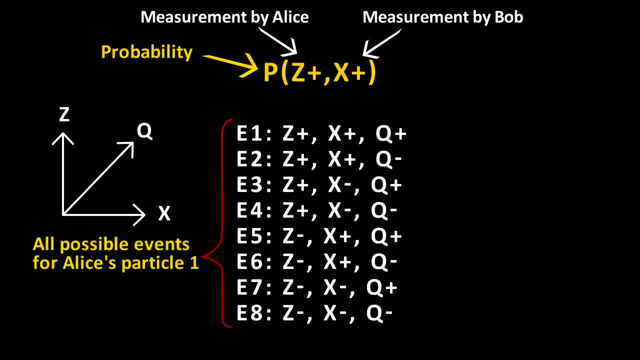 a positive spin and Bob measures in the x direction and gets a positive spin. Well, if the above case is for Alice, there are four events where z is positive. In order for Bob to get x positive, Alice would have to have measured x as negative. So these would 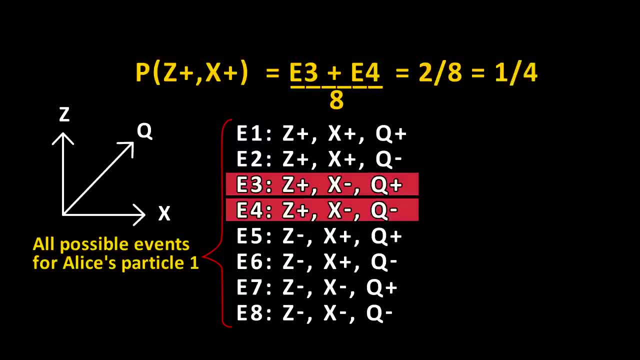 be in events 3 and 4.. To get the probability, we have to divide by the total number of events, which is 8.. Let's do this for two more scenarios. What is the probability that Alice measures positive in the z direction and Bob measures positive in the q direction? In this scenario it would 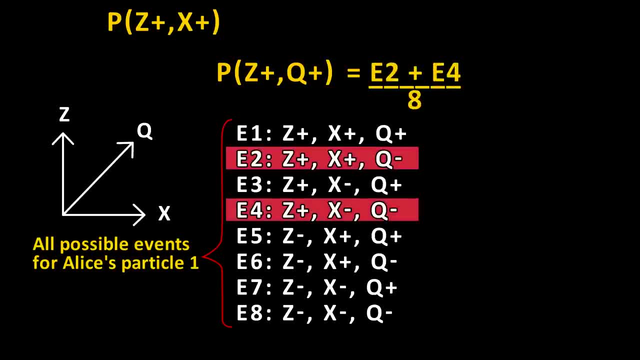 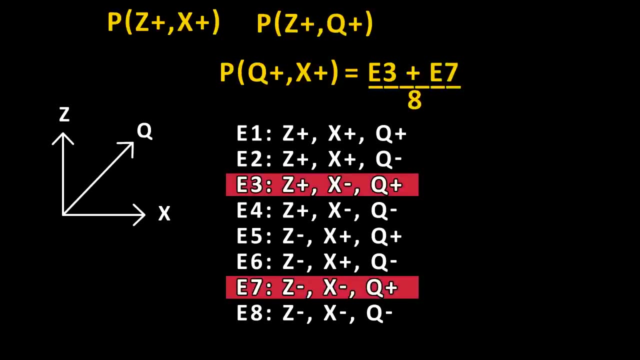 be events 2 and 4. Again, we divide by 8 to get the probability. And the third case is: what is the probability that Alice measures positive in the q direction and Bob measures positive in the x direction? This would be events 3 and 7 divided by 8. 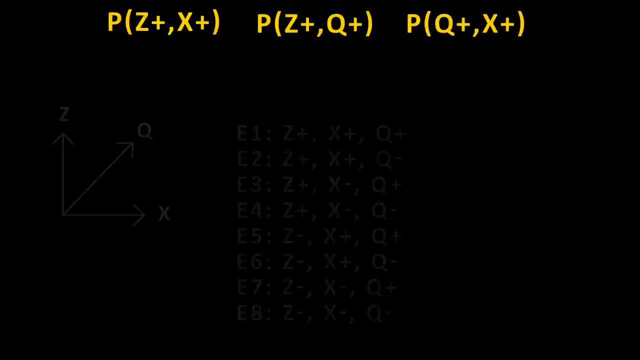 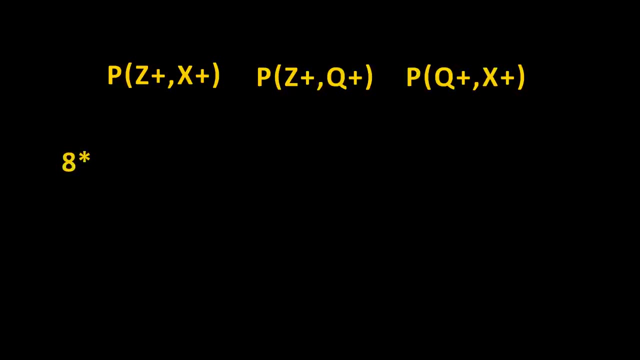 for probability are the three probabilities, given the hidden variables theory. Now here's the big insight that John Bell had: If I take the total number of events and multiply that by the probability that Alice measures Z positive and Bob measures X positive, this has to be less than or equal to the total number of events. 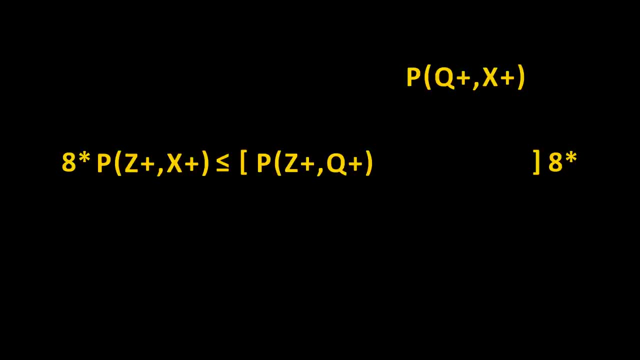 times the probability that Alice measures Z positive and Bob measures Q positive, plus the probability that Alice measures Q positive and Bob measures X positive. When we write this out, the 8 cancels out and we are left with just the probabilities. This is Bell's inequality. Now I can prove this is true. 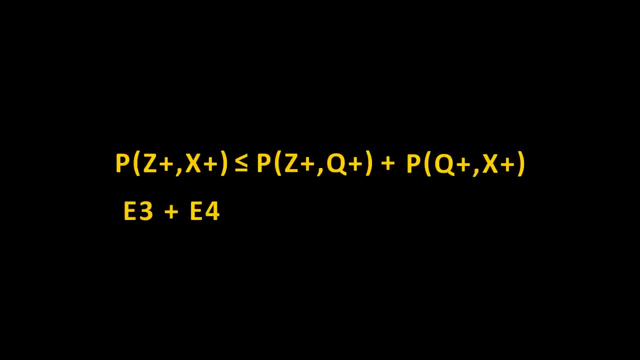 by doing simple math: E3 plus E4 divided by 8 is equal to E2 plus E4 plus E3 plus E7 divided by 8.. The 8's cancel out and we rearrange the order of addition and we're left with this: E3 plus E4 is less than or equal to E3 plus E4 plus E2 plus. 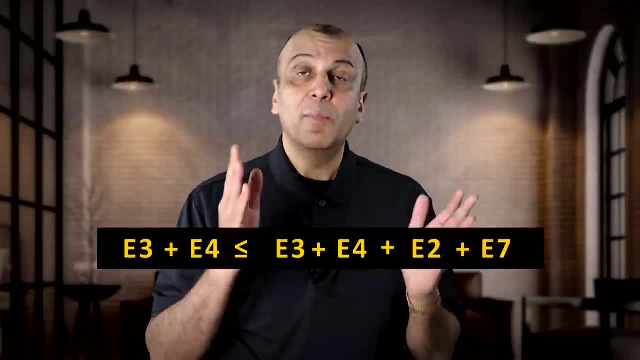 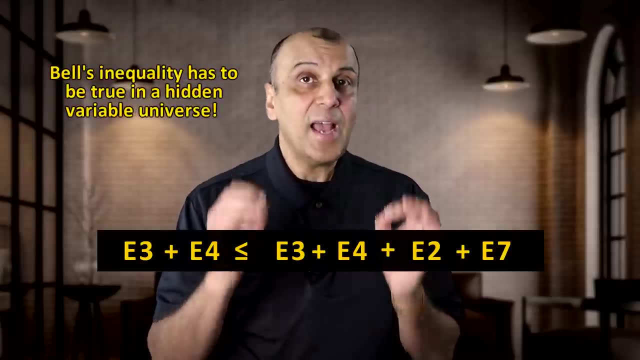 E7. This makes total sense because E3 and E4 are on both sides of the equation and E2 and E7 have to be positive. So this inequality absolutely has to be true for any hidden variables theory to be true. Now, remember, these probabilities are for. 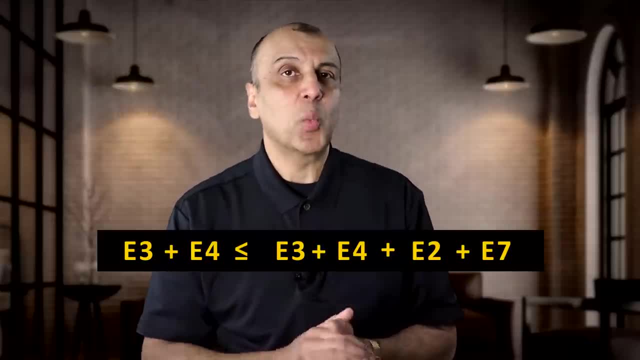 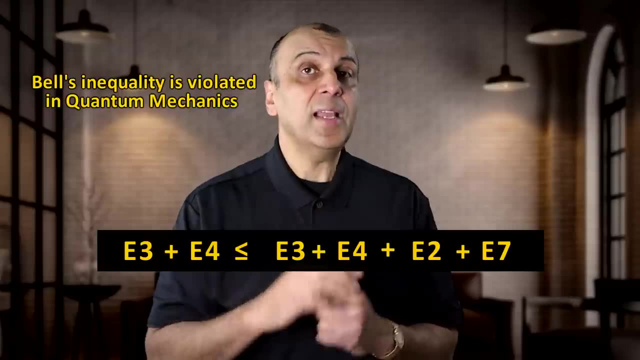 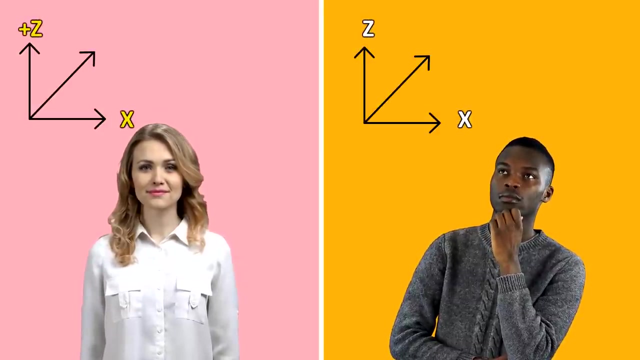 a universe with hidden variables. But what happens in a universe where the laws of quantum mechanics are correct and not the hidden variables theory? Well, this inequality is violated in quantum mechanics. How is it violated? Let's say Alice measures the spin to be positive in the z direction. Then we know that. 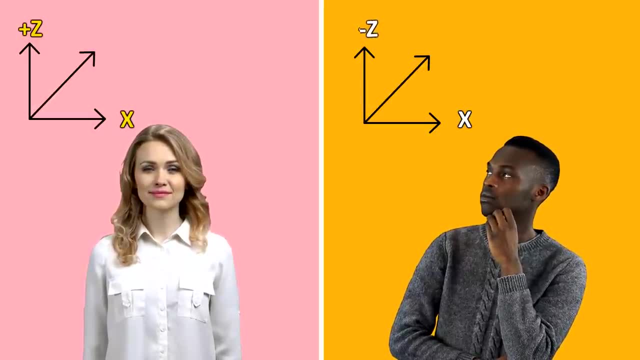 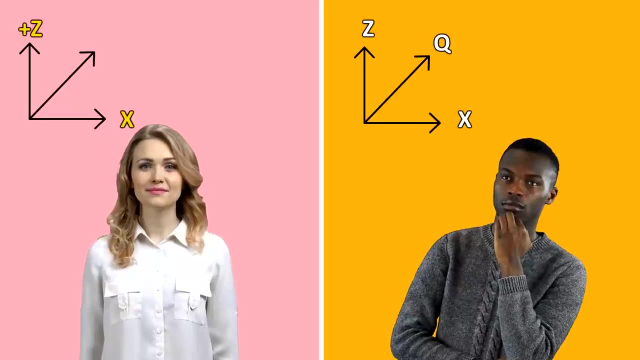 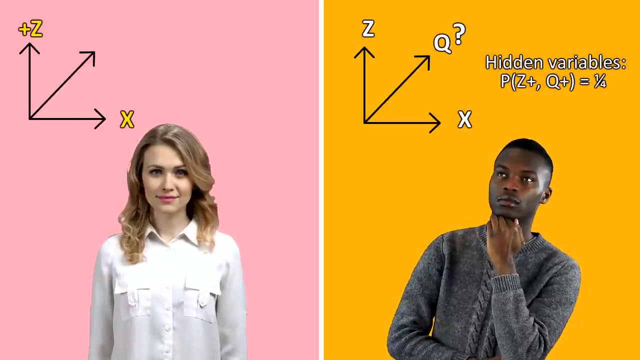 if Bob measured the particle in the z direction, he would get a spin that is negative. However, Bob doesn't measure in the z direction, but in the Q direction. What will the spin of this particle be? In hidden variables there was a 50% chance that it would be positive and a 50% chance that it. 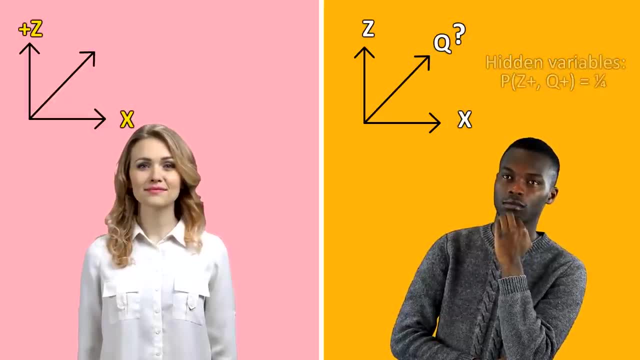 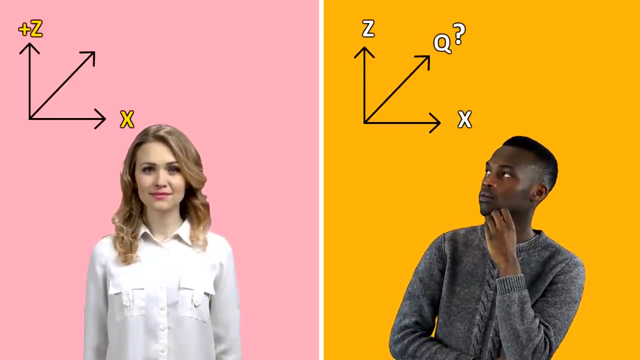 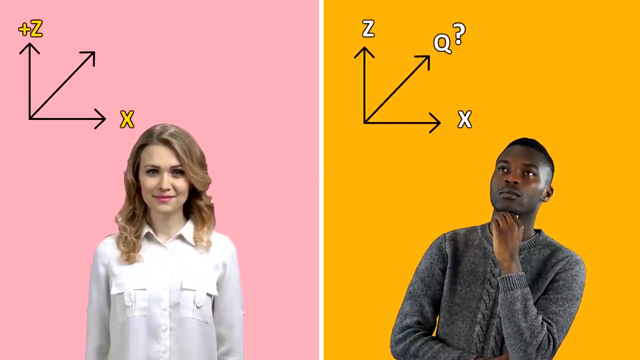 was negative. But this is not what happens in quantum mechanics because the measurement of the particle follows the probability laws of the wave function for a particle rotated 45 degrees And that probability of Bob measuring Q to be positive after Alice has measured C to be positive if the angle between them is 45 degrees. 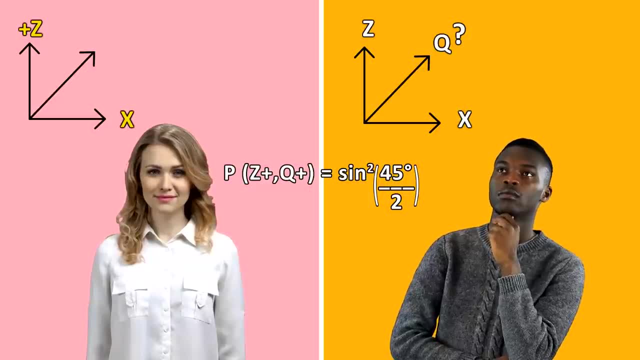 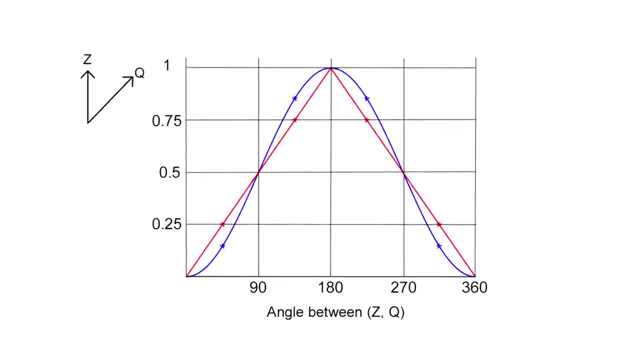 is given by the following equation: Sine squared of 45 degrees divided by 2.. This comes from the math of quantum mechanics. This is the critical difference between quantum mechanics and hidden variables theory. The probability that Bob measures the same spin as Alice, depending. 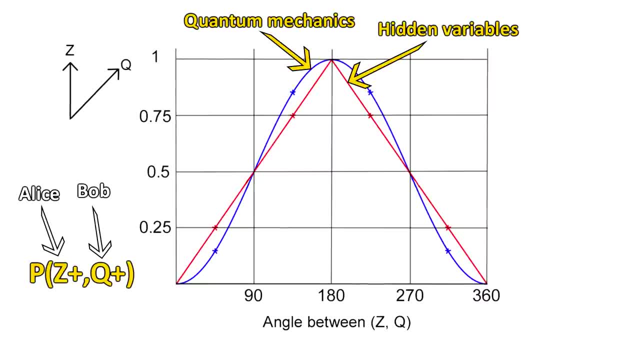 on. the difference in angle measured is not linear but looks like a sine wave. When you plot this out, this is what the probabilities look like. You can see from this graph that at zero and multiples of 90 degrees the two systems are in agreement. But in between, 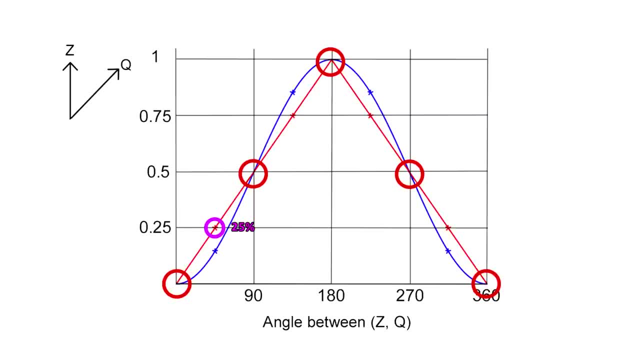 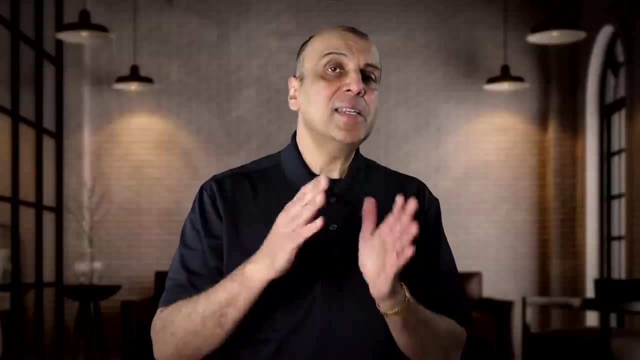 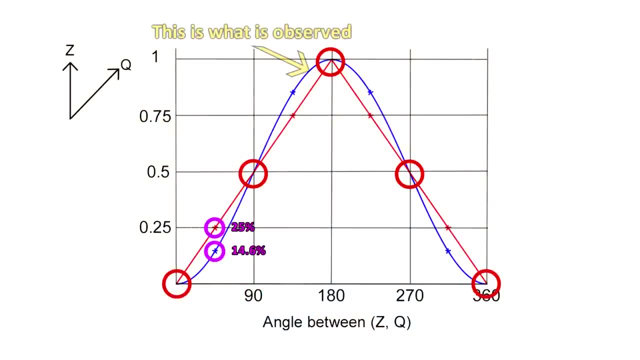 like at 45 degrees. the probability is 25% for hidden variables and about 14.6% for quantum mechanics. But the proof is in the pudding, because in test after test the sine function correlation has been confirmed. The particle does not behave linearly, and so the hidden variables theory. 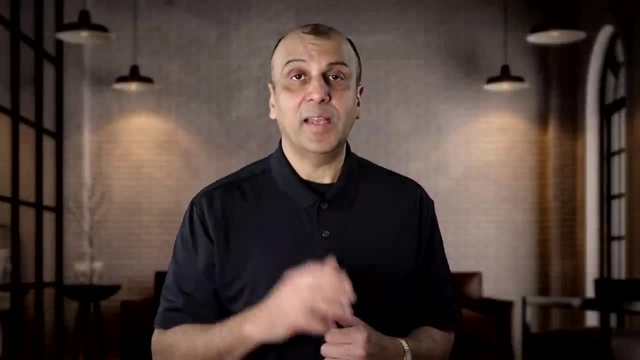 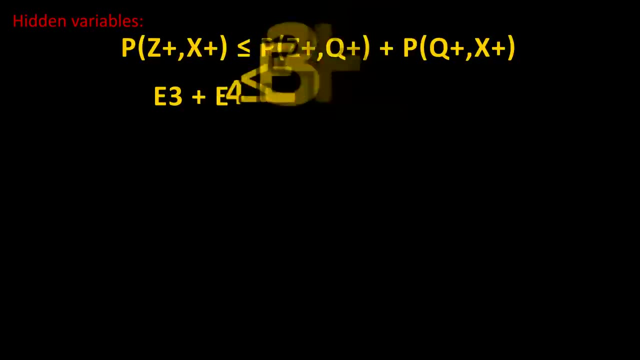 cannot be correct. Bell's inequality is violated. So we can write out and compare Bell's inequality for both cases. For hidden variables, the equation would be: E3 plus E4 is less than or equal to E3 plus E4 plus E2 plus E7.. 2 is less than or equal to. 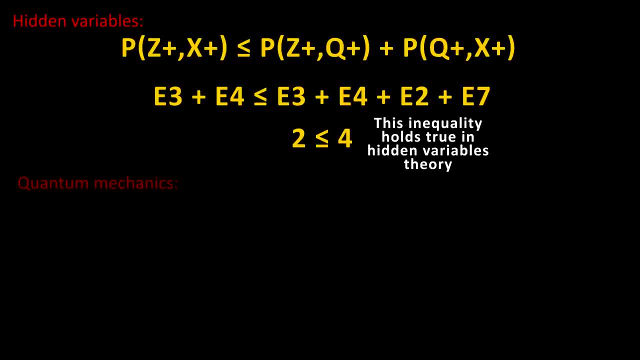 4. The inequality holds True For quantum mechanics. the equation would be: sine squared of 90 degrees divided by 2 is less than or equal to the sine squared of 45 degrees divided by 2, plus the sine squared of 45 degrees. 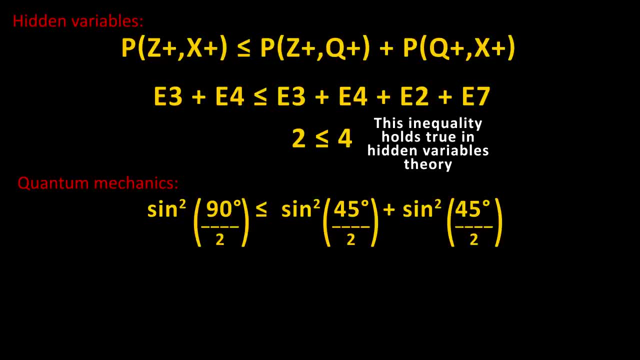 divided by 2.. And when you solve this you get 0.5 is less than or equal to 0.293,, which of course, is not true. So Bell's inequality is violated in quantum mechanics, which is exactly what we observe. 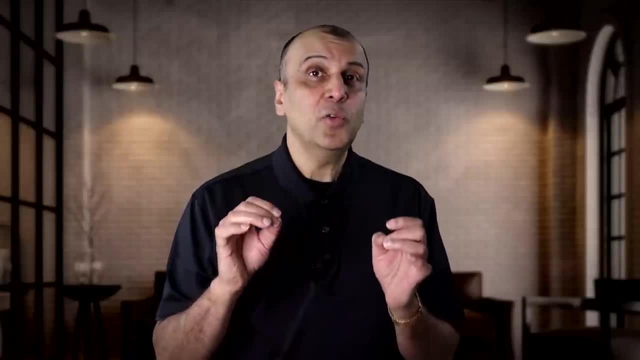 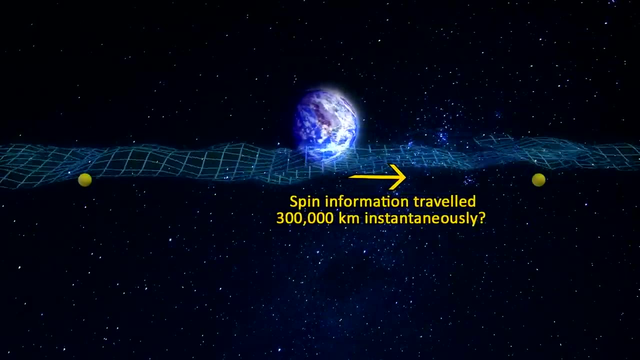 in experiment after experiment. Now, does this prove that the two entangled particles are communicating faster than light? There is differing opinion on this. On the surface it does appear that superluminal communications is taking place, But my personal opinion is that no communication. 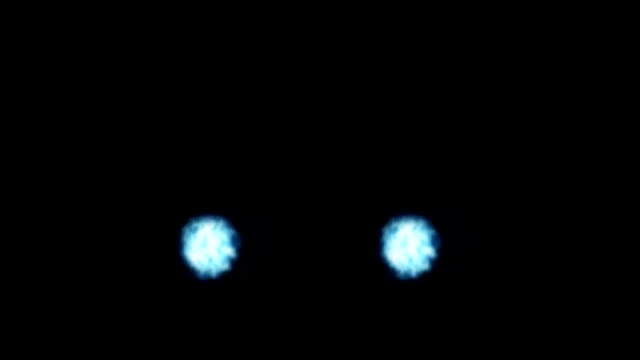 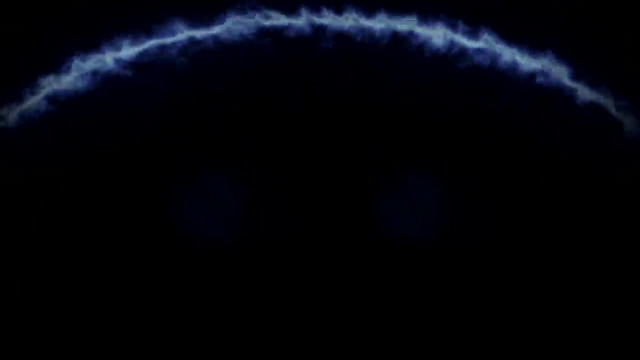 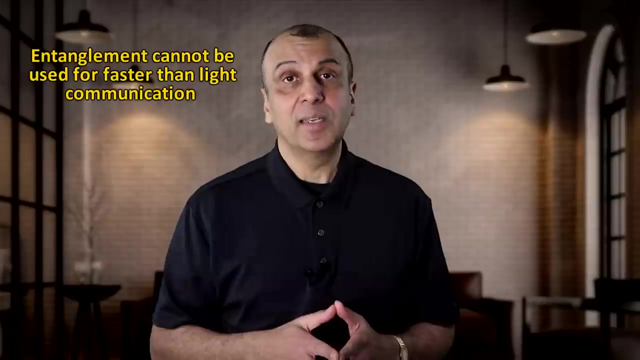 is happening. The two particles are really just part of one wave function And since the wave function can theoretically be as wide as the universe, when this one wave function collapses, both particles collapse And since the collapse is random, it cannot be used to communicate in this way. 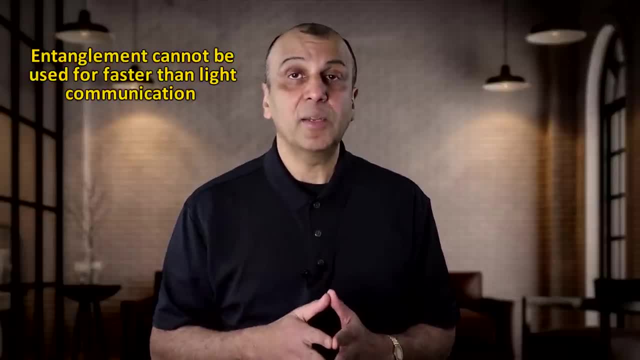 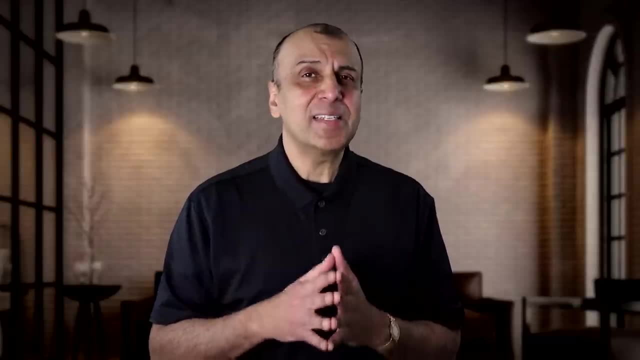 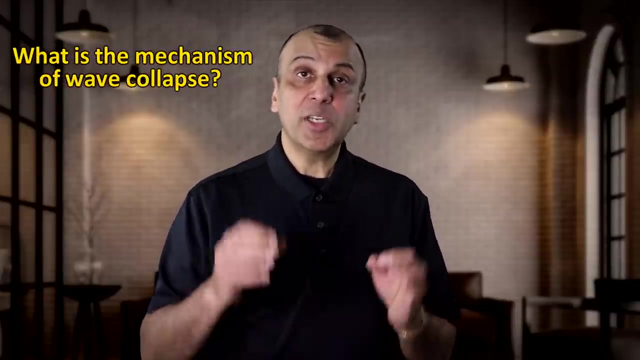 So most theorists do not think special relativity is violated because we can't communicate using this seemingly faster than light phenomenon. But our knowledge of quantum mechanics and entanglement is incomplete, to say the least. Why is there superposition? What is the mechanism of wave collapse between two particles separated? 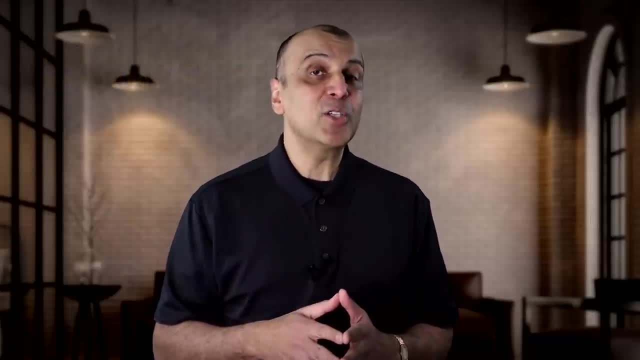 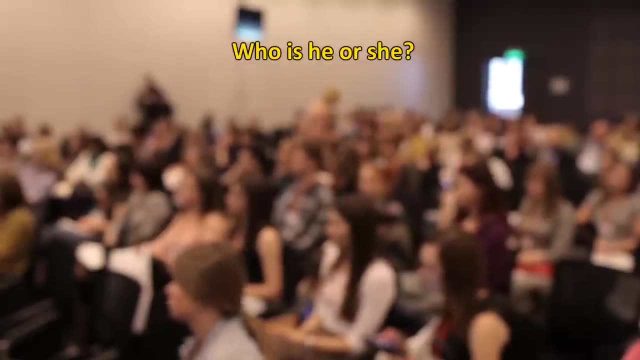 by space and time. I happen to think that the scientist who is going to reveal the mystery of quantum mechanics is alive right now in the world, And I can't wait for him or her to explain this and, like Copernicus, Newton and Einstein, completely change our paradigm. 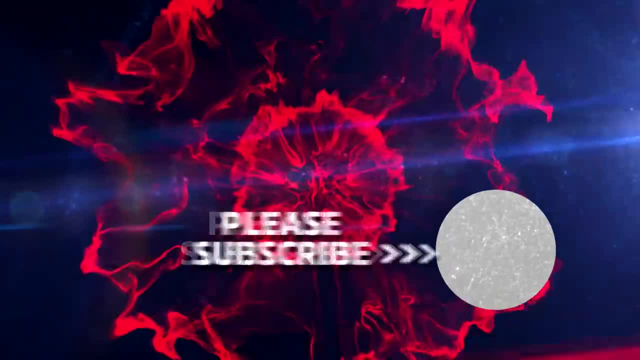 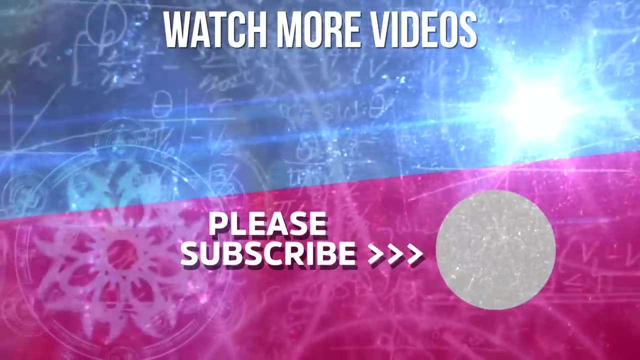 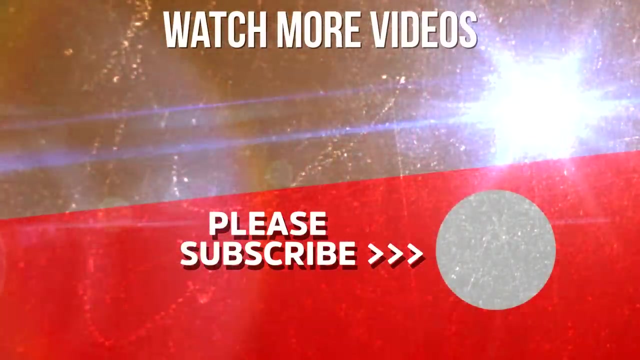 I'll see you in the next video, my friend. Thanks for watching.